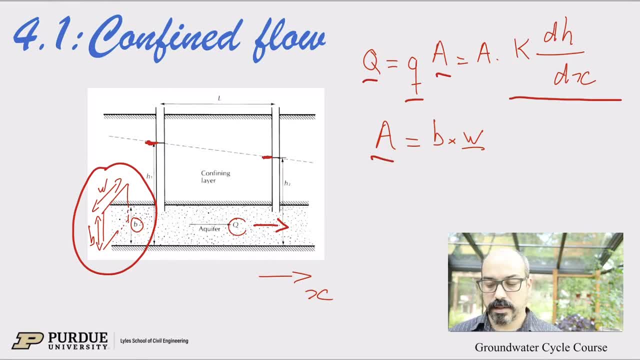 We have the area defined. Of course, Q is the Darcy's law, so it's k, dh, dx, And now we can derive the equations we want. Okay, so if we normalize the discharge by the width, right, we get that Q prime, which is Q over W, which is the Darcy flux times, the depth, okay. 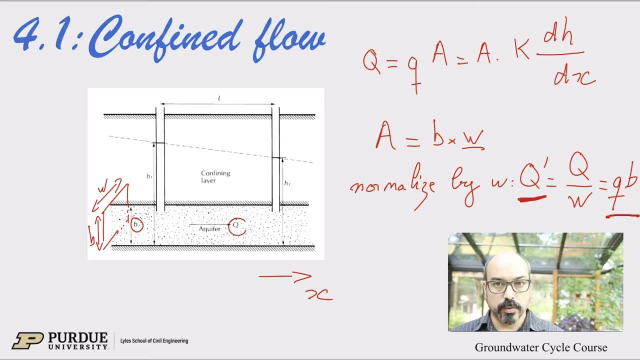 So that means we're going to get flow right Q, but in units of cubic meters per second, per kilometers of aquifer right. So it's per width of aquifer, per you know mile of aquifer. So we get some discharge, but normalized by width, right per kilometer of aquifer. 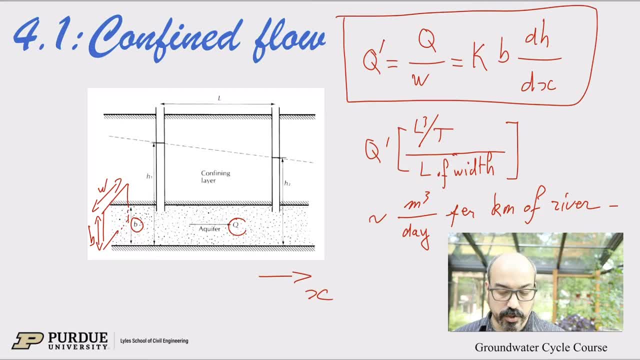 So this is what I'm restating here, right? So you can see the units. If we take the units of Q, prime, right, it's in length, cubed per time, So let's say cubic meters per day, or, you know, million gallons per day. 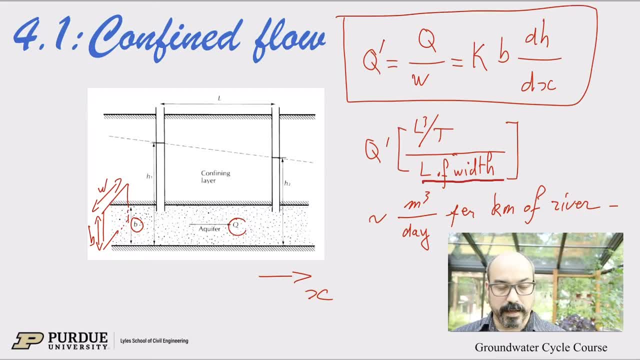 or whatever units you want to put, per length of width, right length of that W unit. So if there's a river, for example, that can be per kilometer of river, right, Okay, So imagine there's a river going across the page here, right? 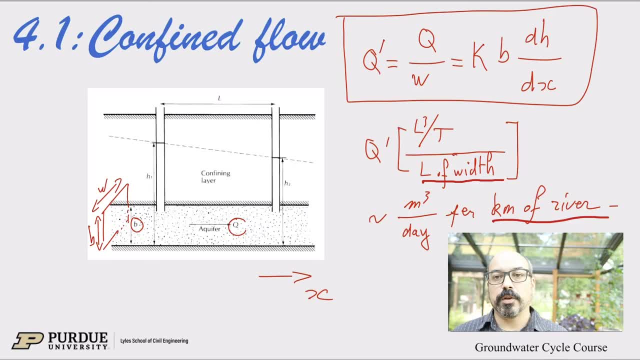 draining that aquifer or the aquifer draining into that river. That would be, you know, the recharge of the river or the discharge of the aquifer into the river per kilometer of river right. So let's say it's a million cubic meters per day per river mile, okay, 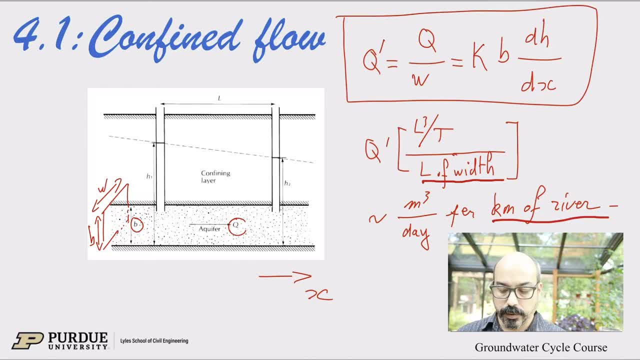 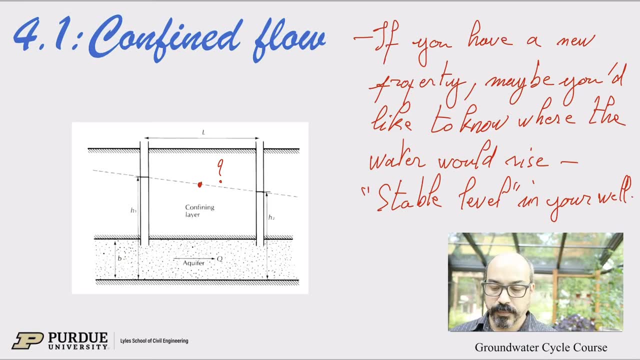 So just to set that up, because we're using this Q prime a lot in the following derivations: Okay, So let's say you have, Let's say you have a new property and you'd like to know where the water would rise, right? 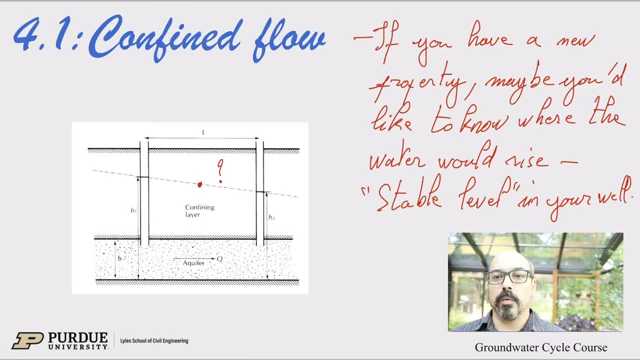 Let's say you have a new property and you want to put a well right and you don't know what the stable level in that well would be. So well, maybe you want to calculate that. This is what these equations we're deriving now can be used for. 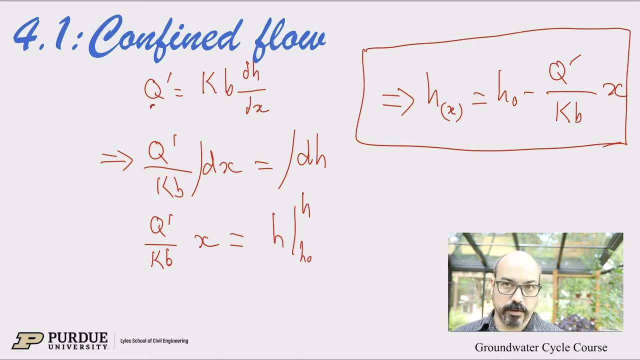 Okay, So, as we said before, we know that Q prime is, you know, the hydraulic conductivity K times the depth of the aquifer. Again a constant for a confined aquifer. So let's say we're going to take the 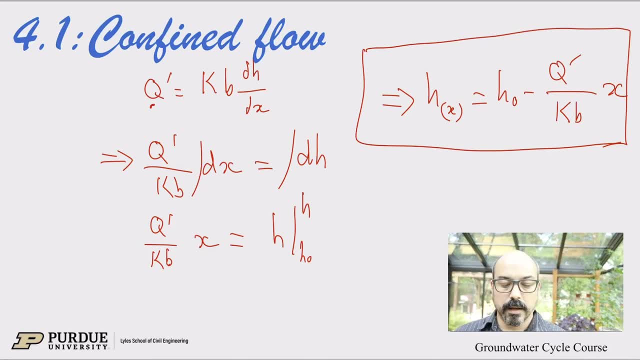 the hydraulic conductivity K times the height gradient, dH, dx. Okay, Well, now we can separate the variables, integrate on both sides. So separate the variables right here. So put dH on one side, dX on the other side. 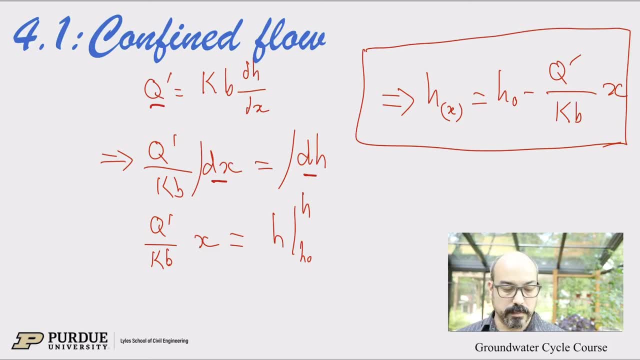 Everything else is basically some constants, right, So we can just throw them together. So Q prime divided by KB. We put dx on the left-hand side and now we integrate both sides. Of course the integral of dx is x. integral of dH is h. 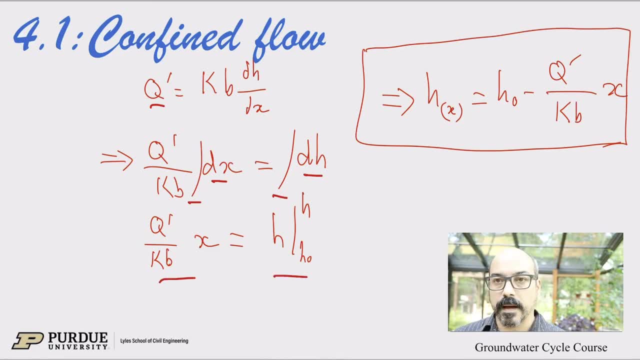 So that gives us a pretty simple, a pretty simple equation, right, So x between 0 and x, So at 0, it's just 0, so we don't count it. And then h between, you know, h0 and h1,. 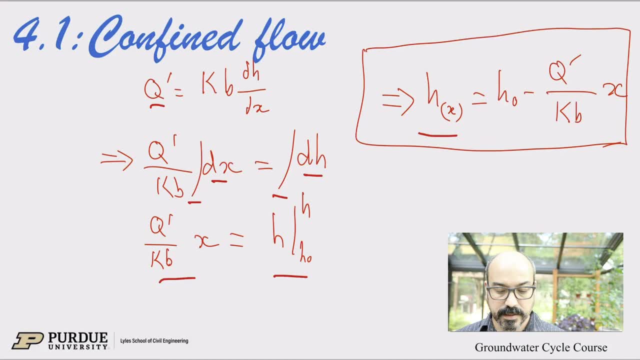 or whatever the boundaries are. so that gives us h of x equals the initial, you know, h minus Q, prime over KB x. Okay, So a pretty simple equation. Now we can calculate the head anywhere right between the two wells. 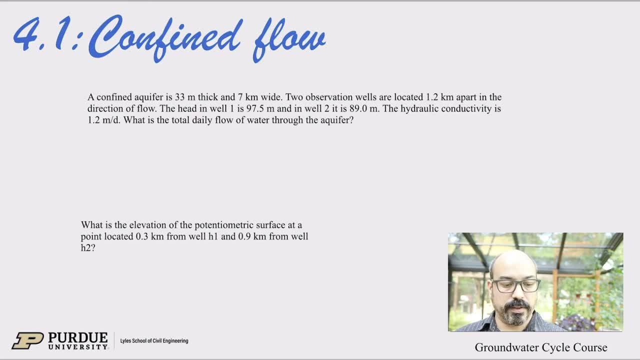 So, for example, if the confined aquifer is 30,, 3 meters thick and 7 meters kilometers wide, right two observation wells are located 1.2 kilometers apart in the direction of the flow. the head in the well is 97.5. 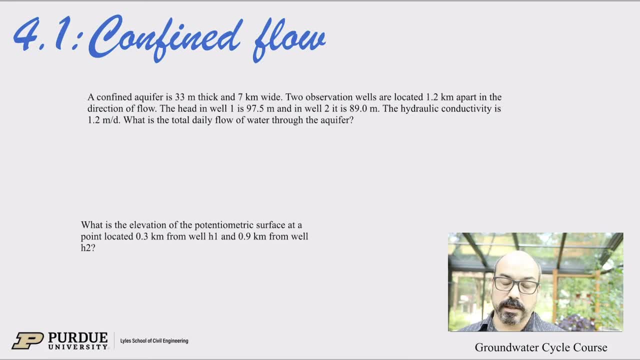 and in another is 89, right where the hydraulic conductivity is given at 1.2 meters per day. That's a pretty standard number for hydraulic conductivity. Again, remember, meter per day is a good approximation. What is the total daily flow of water through the aquifer? 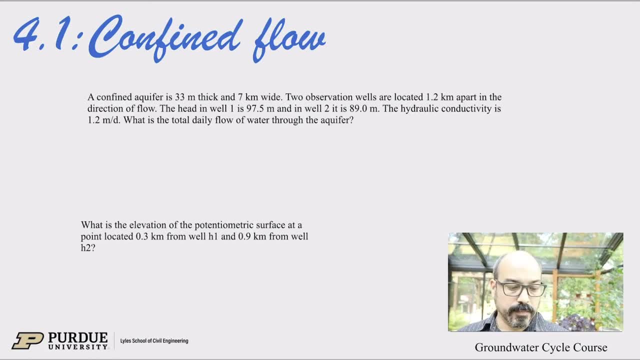 So that gives us? you know how much water flows through the aquifer. What is the elevation of the potentiometric surface at a point located 0.3 kilometers from the first well and 0.9 from the second one? So let's say this is where you're thinking of putting a well right? 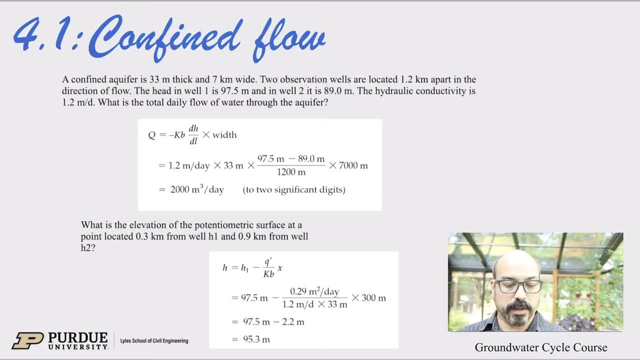 for your property. well, what is the stable level in that? well, Well, you can just plug these numbers right in those equations that I just gave you. So Q, the total discharge, that's the question, right? not Q? prime, not Q. 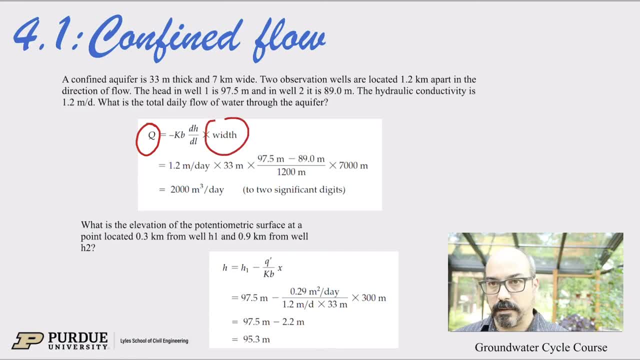 So you have to multiply by the widths which is given. but it's still our same equation, right? it's Darcy flow times the depth, right? and then you plug it in, And then you plug in all those numbers and you find that this is an aquifer.